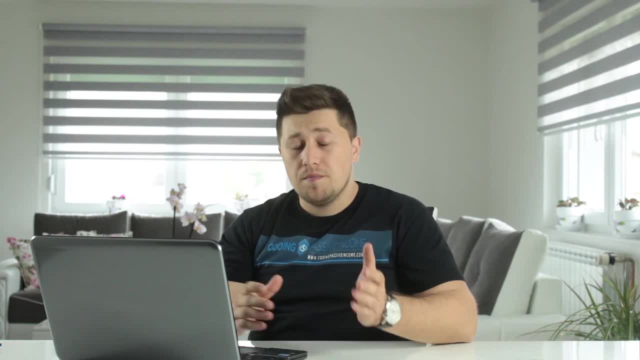 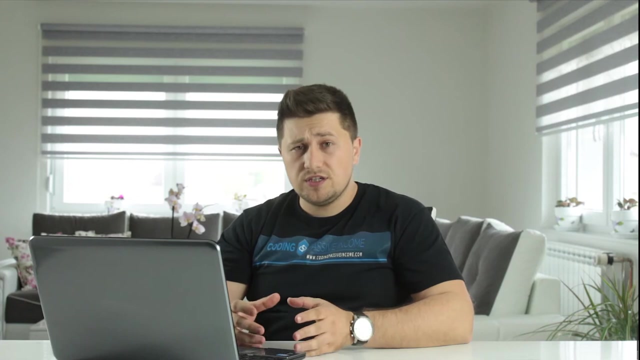 the place where I help others to become a web developer much easier and faster than they will do it on their own. So if that is something that interests you, consider subscribing Now. for some of you that don't know, cross-site request forgery is an attack where a malicious 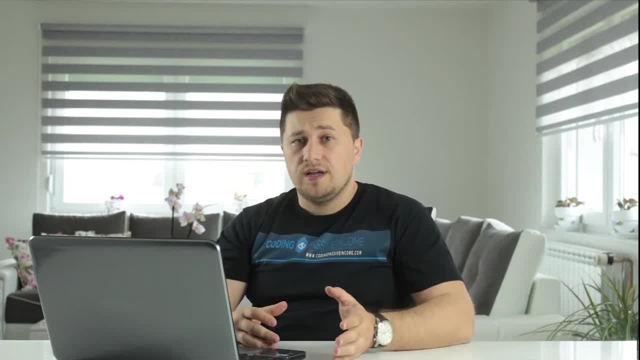 website will send a request to a web application that a user is already authenticated from a very different website. This way, an attacker can access functionality in a target web application where the victim is already authenticated. Target web applications include web applications like social media, in-browser email clients. 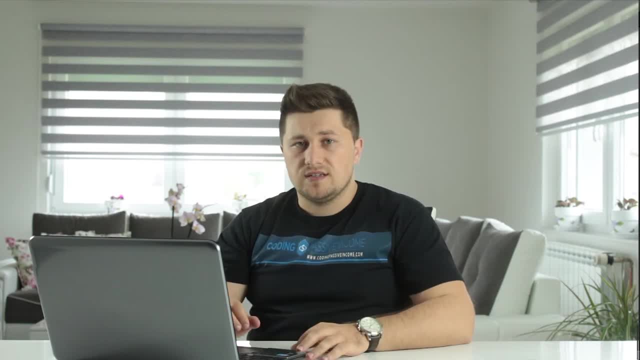 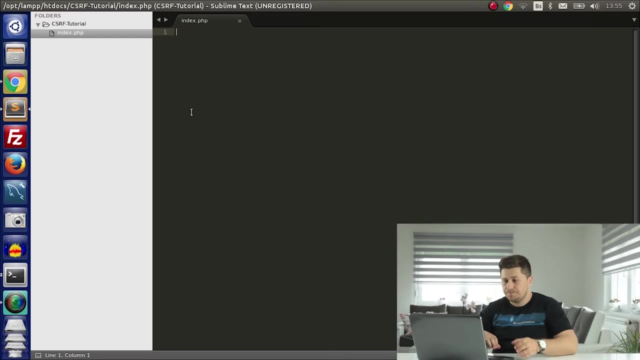 online banking and web interfaces for network devices. This is a very simple explanation, and I hope so that this explanation will give you the basic understanding. what is cross-site request forgery? Now let me show you how to implement protection in PHP. So now I'm here at my sublime text and I 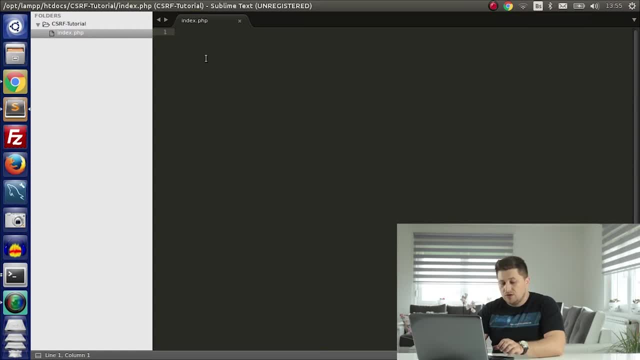 just want to show you how to implement protection in PHP. So now I'm here at my sublime text and I just created the normal indexphp file. So, as you can see, first we need to define some PHP code and I'm going to write here what we need to do. So first thing that we need to do is we need to start. 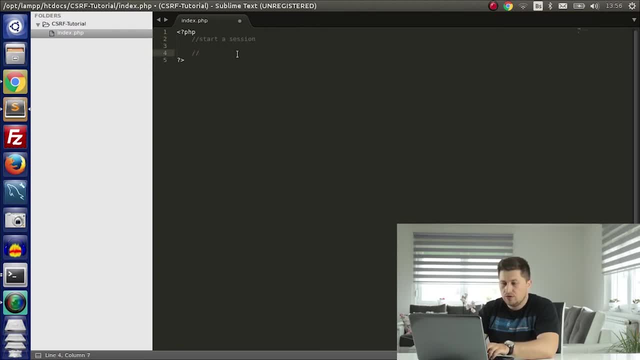 a session. After that, we need to create a key for hash it make function. After that, we need to create ccfi token and the last thing that we need to do is we need to accept the information from the form that we will create in HTML and validate the token. So we need to validate the 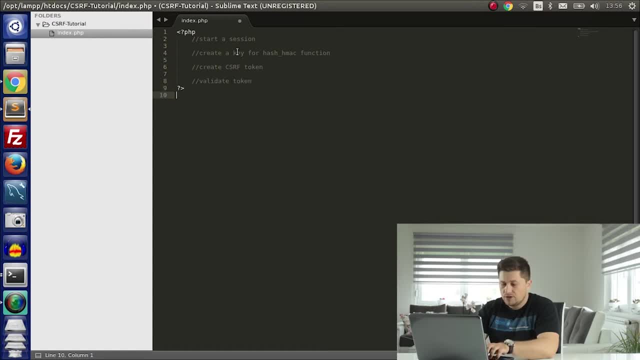 topic. Okay so I'm going just to create some basic HTML form, nothing special. Okay, so I will say here: form method will be post and action will be indexphp, which is the same file. Okay, so I will say here: form method will be post and action will be indexphp, which is the same file. 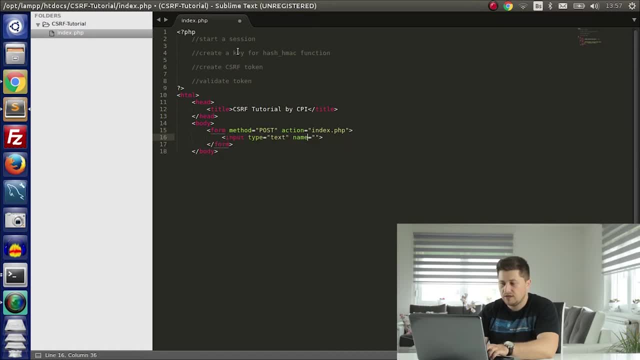 So we will just have one input type will be text name, will be username, username and the placeholder will be what is your name? very simple. we will have one hidden button. we will store our CCR5 token, okay, and we will have one submit button. 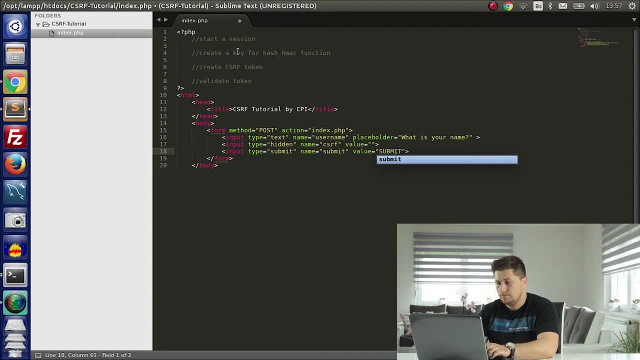 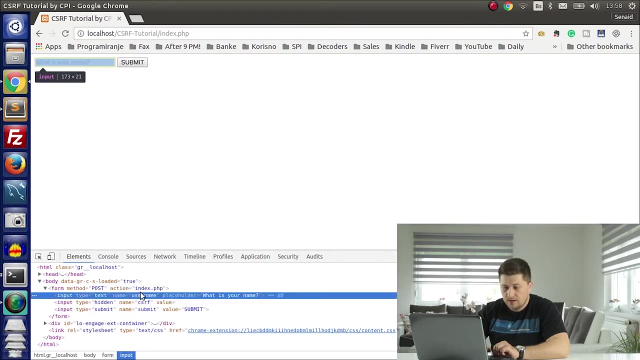 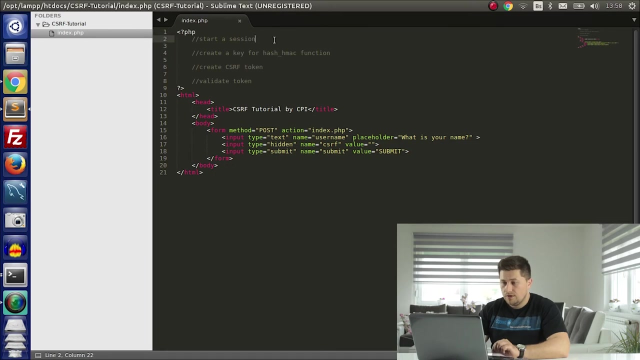 you, okay? so this is one very simple HTML4. let's now just see so and see we have two inputs- one is here and one's type text- and then press submit. nothing happens. you should already know that. so now we need to start our session. okay, I am going to close the session. 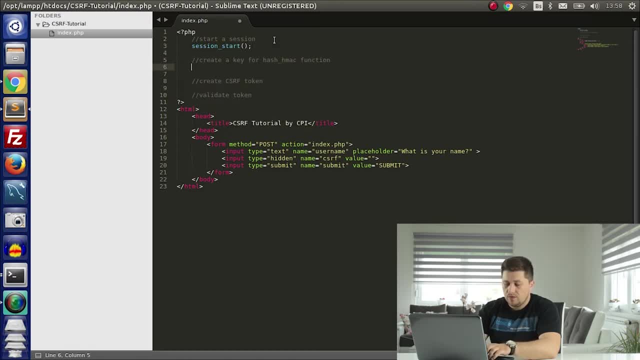 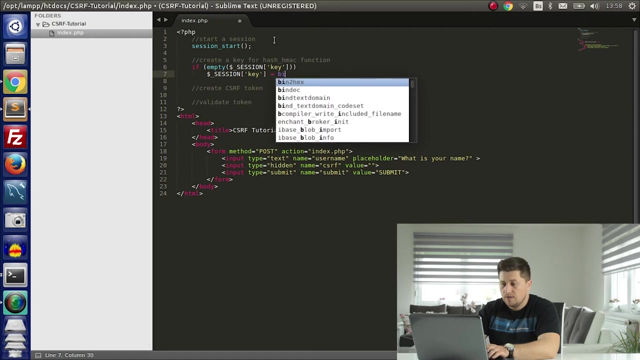 after that we want to see: do we have already created our session? so if we are not, we will create new key that we will use for hash HMAC function. and I'm going to create by calling two functions: first, binary to hex, and there I will use random bytes and I will use 32. so, as you can see, this function will create 32. 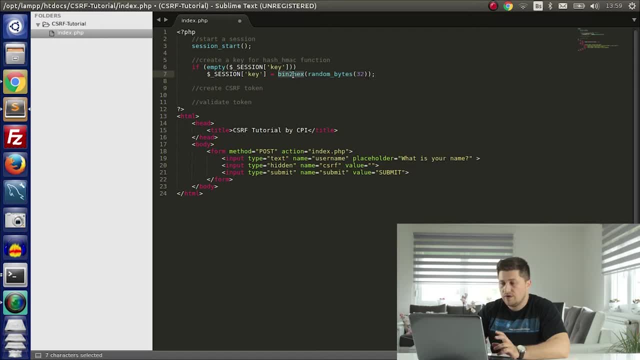 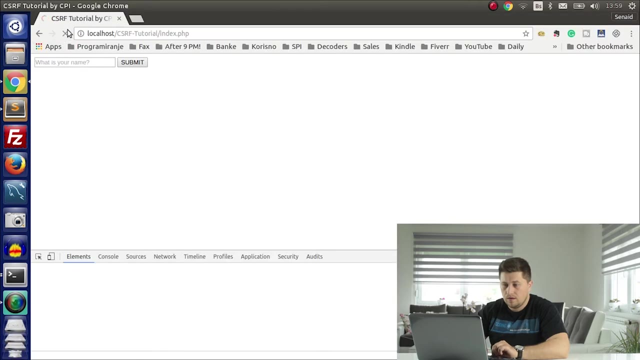 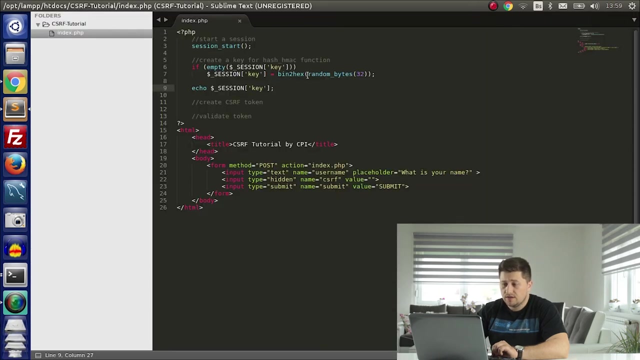 random bytes, and this one will convert that bytes into the hex format, so we can see what we got by using this. that's it and it is. we are saving this hash into the session because we want to be sure that our key is always the same, or otherwise we won't be able to validate our CCR5. 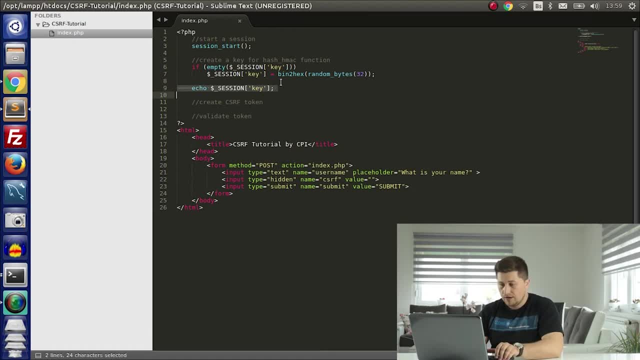 token. that is inside the form. okay, now the next thing is we need to create our CCR5 token. we will do that by doing by calling hash HMAC function. the type of the encryption that I prefer to use is 256 for the data. we can write any type of the string, but what I usually do is I'll write some string and 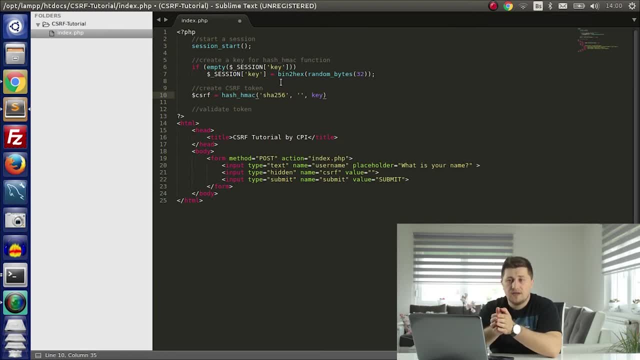 at the end of that string I will append the name of the current file. that helps me so that if I have ten different files, on every file I will have a different CCR5 token. so let's write the see I. Here in this file is the 휴대 Ifér. 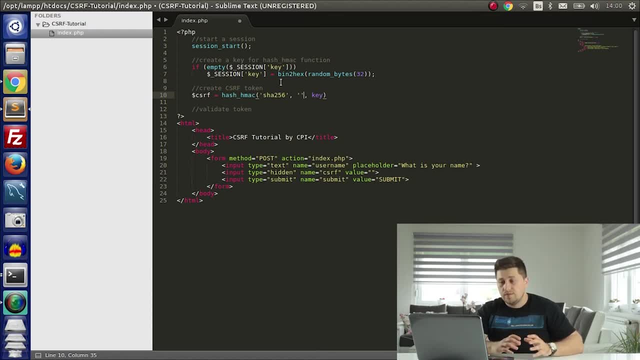 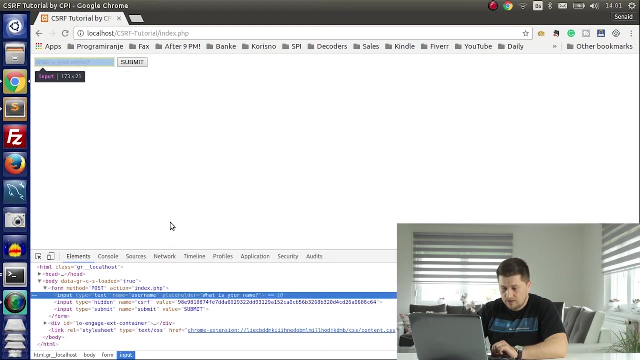 that way we have protected, each time on the different way, our form. so I will write here: this is some string and I will say index PHP and we have created the key. it's stored inside the session. it does say key and down below we need to output this: CCR 5 talk. let's not test. we take this as you can see, here we 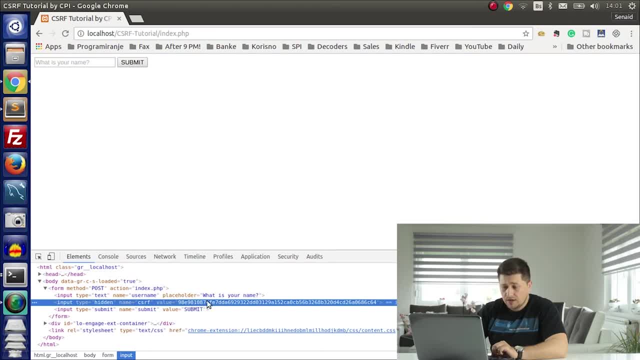 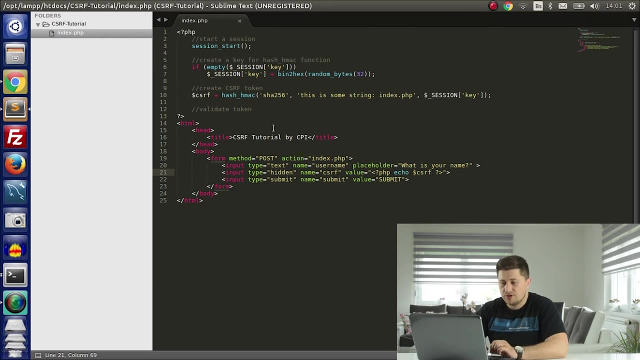 have our Caesar fight talk, which is a very long token, and it's almost not possible to guess this string because we are using some very powerful functions that are available only in the program PHP 7 version. so the next thing is: we need to validate token. so first thing is: 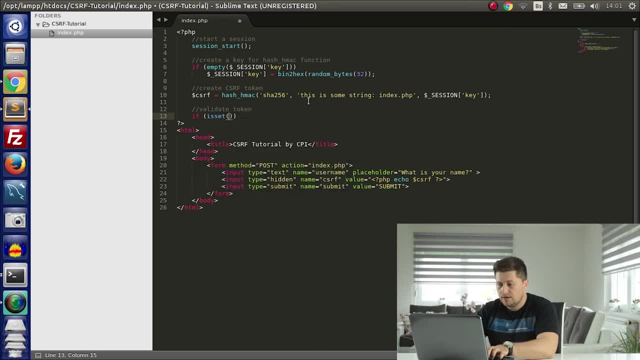 we are going to do is if test set, post submit, which means this part of the code here will execute only if this button is pressed. so here we need to verify our token. I I can do something like this: CCR 5, equal post CCR 5, but that is not good enough protection. so I want to do: